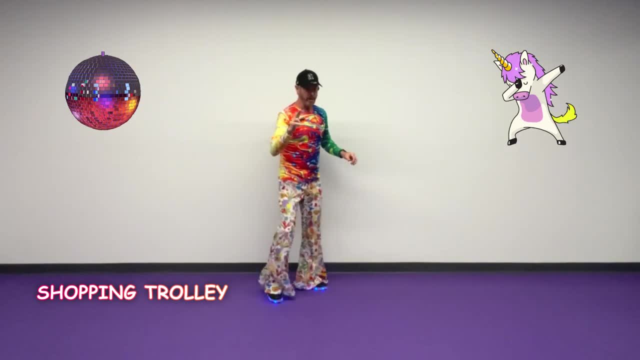 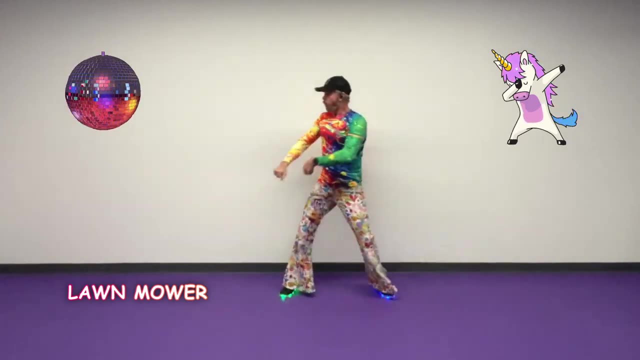 We'd better get outside and mow the lawn. We've got our lawn mower, We've got to start it up. first of all, One two, one, two, three. One, two, one, two, three, One, two, one. 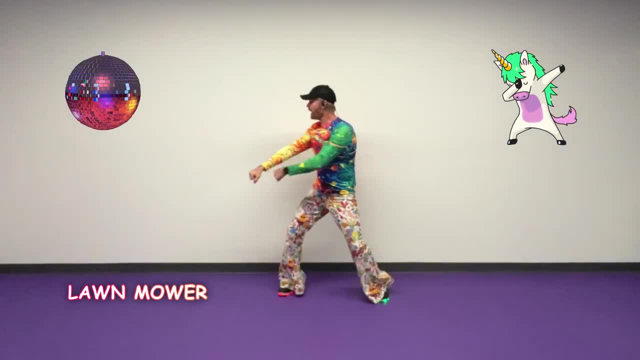 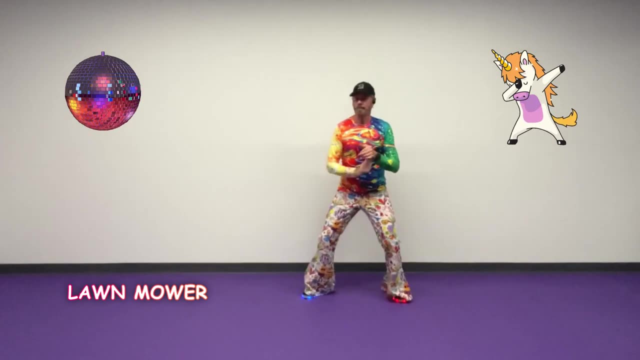 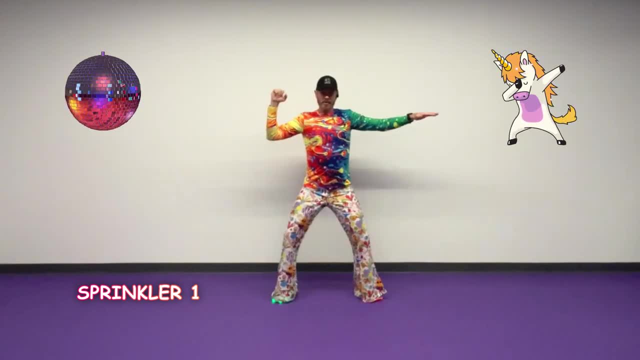 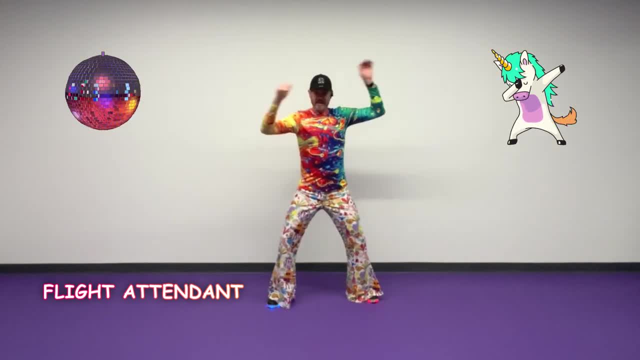 We go exit, exit, facemask, seatbelt, exit, exit, facemask, seatbelt, exit, facemask, seatbelt, facemask. Speed it up. One, two, three, four, hey. 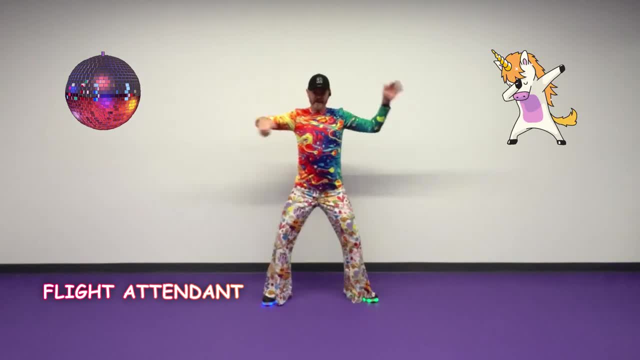 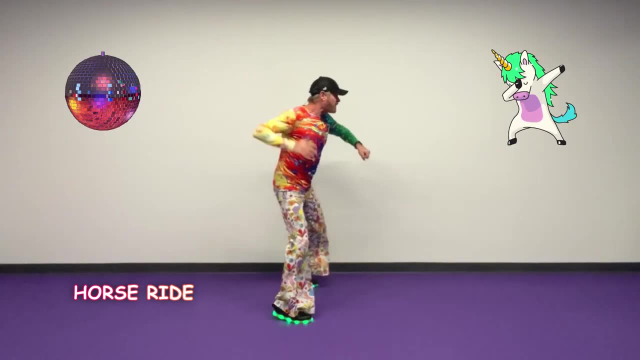 Exit, exit, Let's ride a horse. Three, four, five, six turn with me. One, two, three, four, five, six, seven, eight. Hey, two, three, four, five, six, seven, eight.